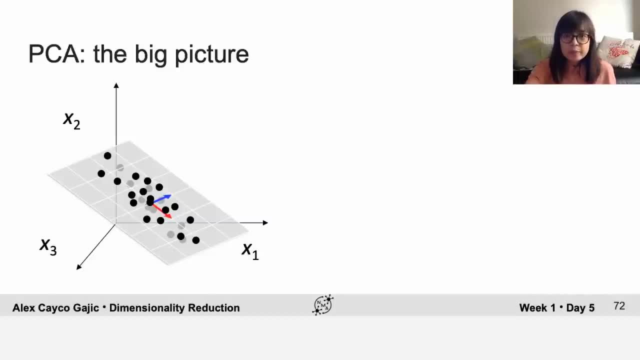 of the variability in your data. We often call the subspace that's generated by this basis the latent subspace, and, after the transformation, we often call this the latent representation. Latent means hidden, because these components are not directly observed in the data, but they're. 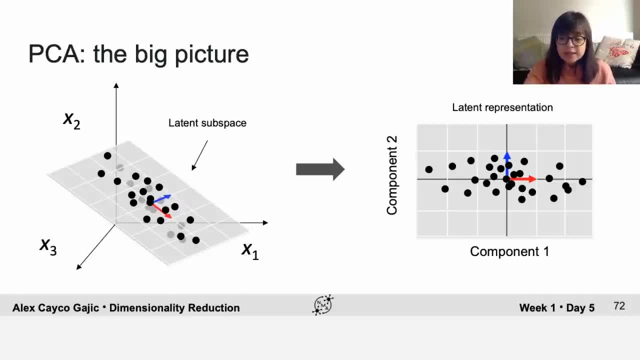 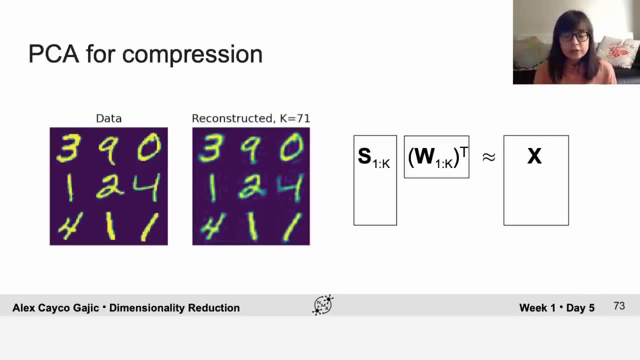 inferred from the structure, PCA has a number of different applications and I'll go through four that are very useful. So, first of all, PCA, as you saw in the last tutorial, can be used for compression. That's related to the fact that PCA has an alternate formulation as finding the low. 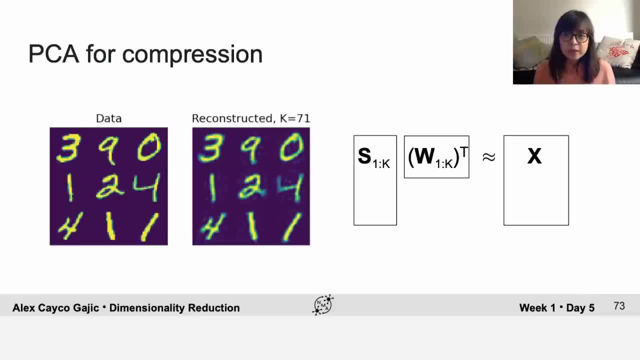 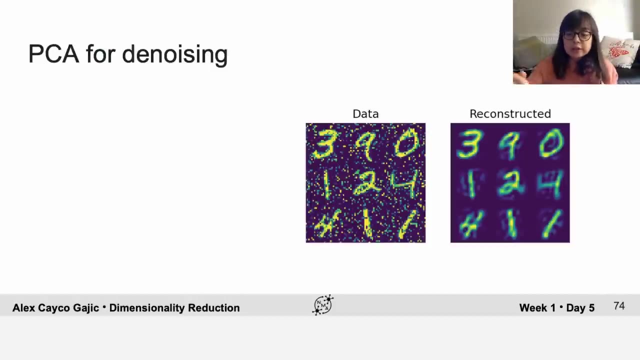 dimensional basis that minimizes the reconstruction error. So instead of saving your full data matrix x, you can save the data matrix x. PCA can be used for denoising. You saw this also in the last tutorial. So to understand this a little more intuitively, we can imagine a data point that's given here in black and I'm going: 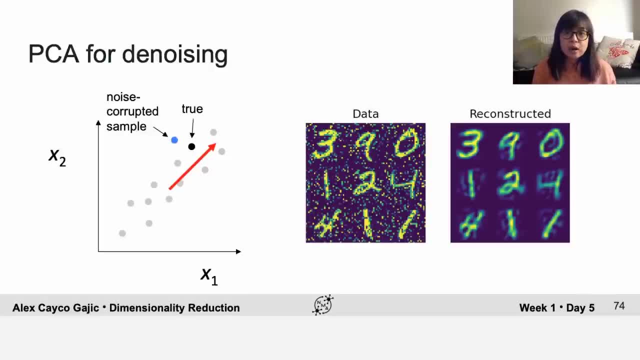 to show you in blue a noise corrupted sample of that same data point. But then when you project onto the low dimensional subspace, you're basically removing any noise that's orthogonal to that subspace. So PCA can also be used for denoising. for this reason, And third, PCA can be very useful. 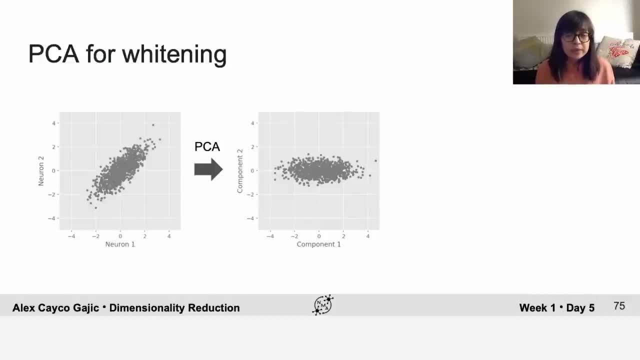 for whitening, which is a procedure in which you de-correlate your data and you standardize it, meaning that you you rescale it so that the individual components have unit variance. And we saw in the first couple of tutorials that PCA finds a transformation so that the 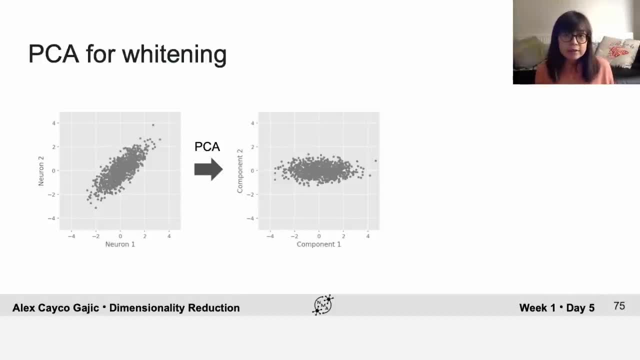 new components are uncorrelated and we know that the variance of each component is given by the eigenvalue. So we can just rescale this so that the new components are uncorrelated and have unit variance. So these first three properties that PCA can be used for. 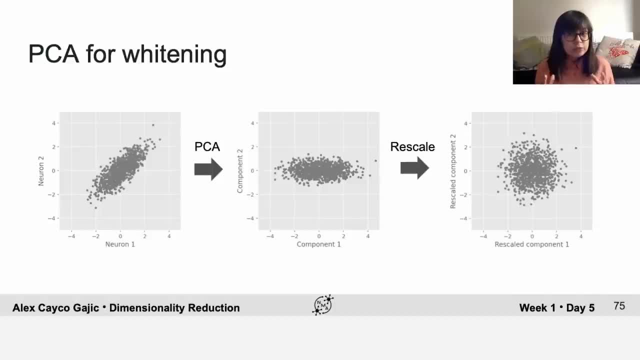 compression, denoising and whitening are extremely useful in a very wide variety of settings and actually, if you want to do a more complicated non-linear dimensionality reduction technique, it's often useful to use PCA as a pre-processing step for exactly these reasons. And the fourth: